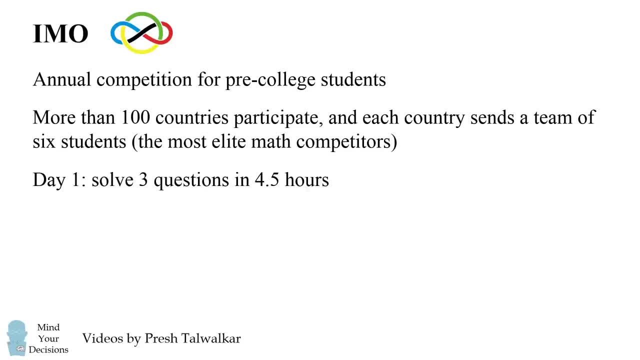 six elite math competitors. On the first day, students solve three questions in four and a half hours, and on the second day, they solve another three questions in four and a half hours. Each problem is worth seven points, for a total of 42 points In 2019, the individual mean score: 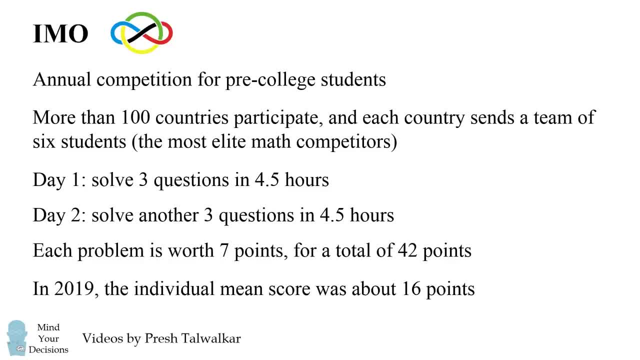 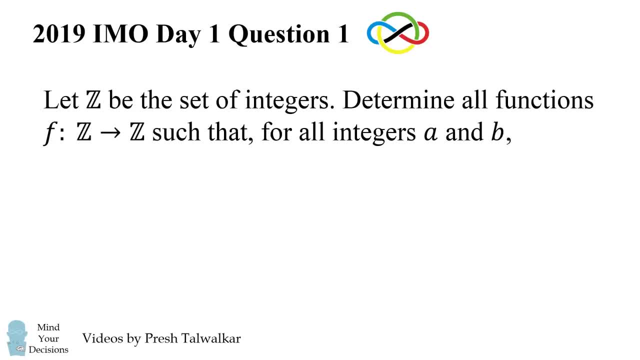 was about 16 points, but there were students who got a perfect paper with 42 points. This problem comes from Day 1, Question 1.. Let Z be the set of integers. Determine all functions f going from z to z, such that for all integers a and b, f of 2a plus 2 times f of b is equal to f. 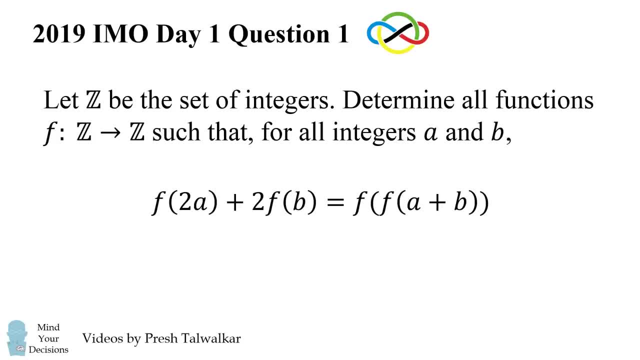 of f, of a plus b. Now, while this is an incredibly challenging problem for most of us, about 60% of these competitors scored a perfect 7 points on this problem. For them this was an easy problem, but for the rest of us this is a very challenging problem and in this video I want to give some 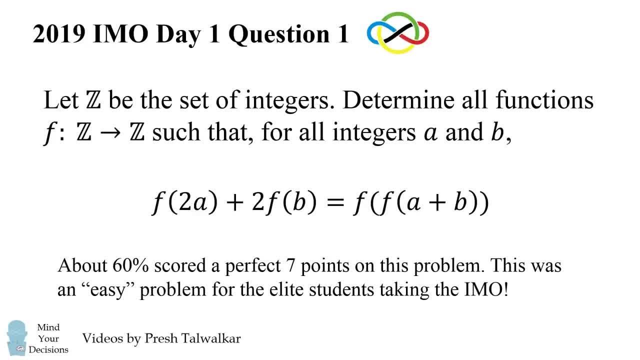 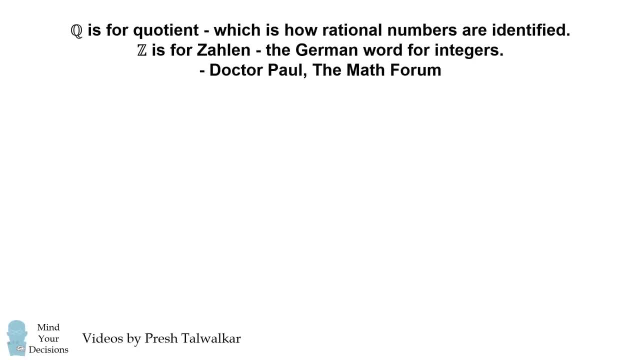 indication of how you can solve it. Pause the video if you'd like to give it a try and, when you're ready, keep watching to learn how to solve this problem. So I'll admit I wasn't able to solve this problem myself. 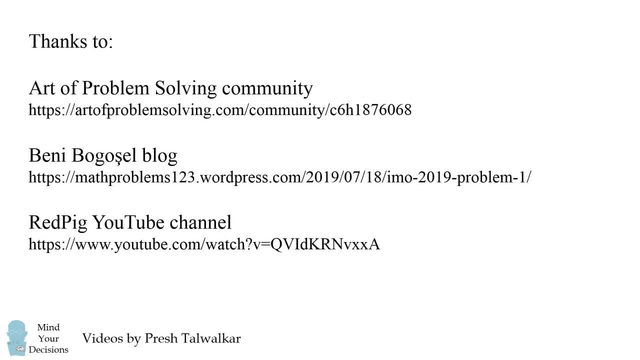 but I want to thank the Art of Problem Solving community, Benny Bogusel's blog and the Red Pig YouTube channel. I read solutions on these places and it helped me understand how to present it for you. So how can we solve for all functions over the integers, such that this: 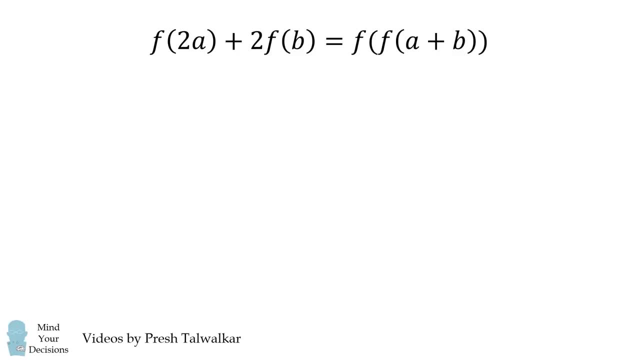 equality is true. Now, solving this problem is a little bit like giving directions from point A to point B. You're going to have to calculate a lot of different routes until you figure out a good way to go from A to B, Just like a GPS will show you the shortest path or a path that's easier to understand. 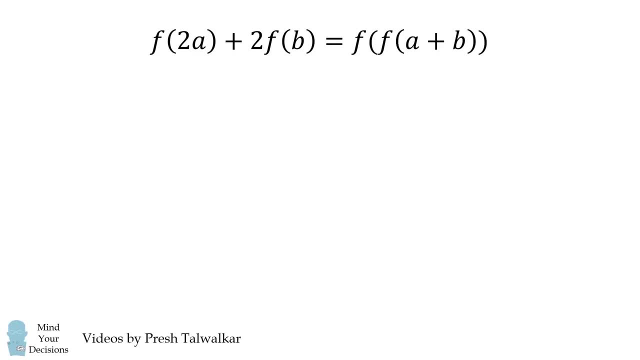 I'm going to just present the solution to you as if we've already done all the experimentation. There may be other, easier ways, but this is just one way that I hope you'll understand. So we'll get started by trying some special values. Suppose A is equal to 0.. We'll take 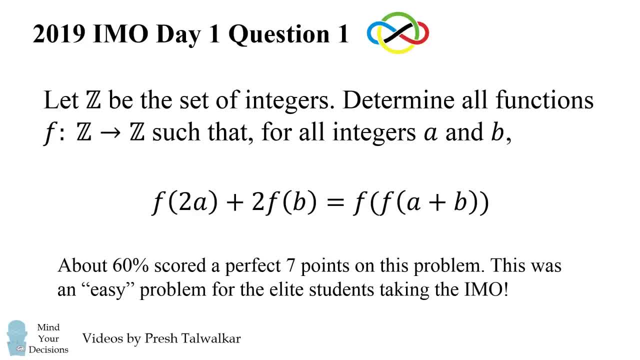 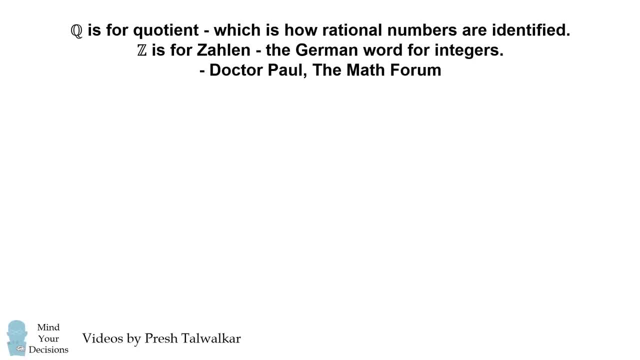 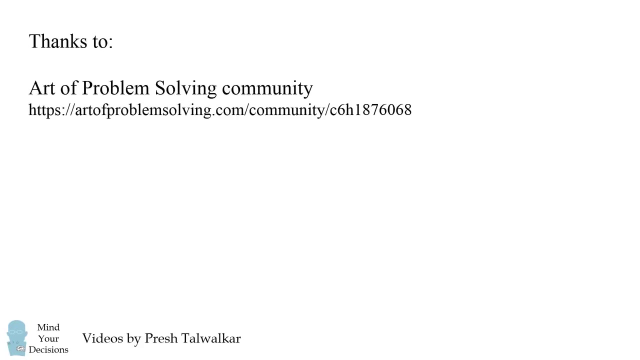 indication of how you can solve it. Pause the video if you'd like to give it a try and, when you're ready, keep watching to learn how to solve this problem. So I'll admit I wasn't able to solve this problem myself, So I want to thank the Art of Problem Solving community, Benny Bogusel's blog and the Red Pig YouTube channel. 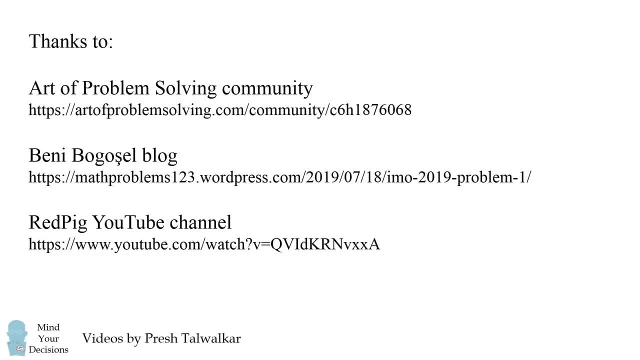 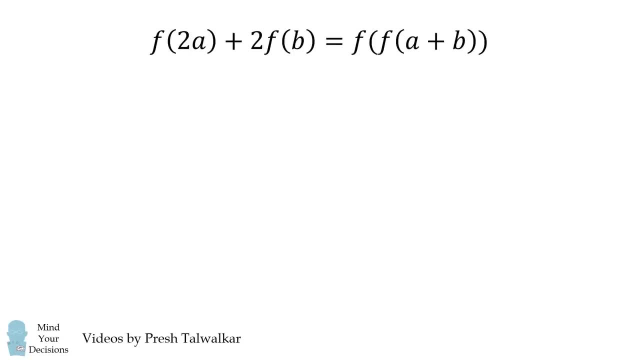 I read solutions on these places and it helped me understand how to present it for you. So how can we solve for all functions over the integers, such that this equality is true? Now, solving this problem is a little bit like giving directions from point A to point B. 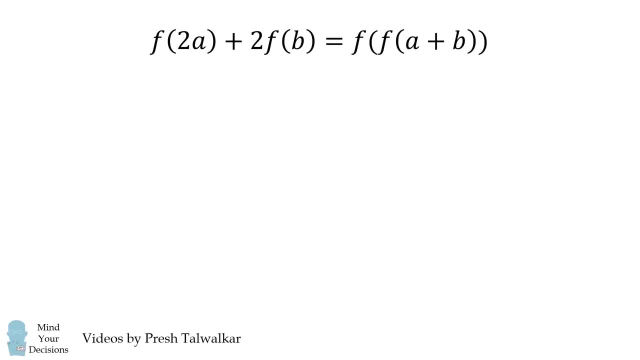 You're gonna have to calculate a lot of different routes until you figure out a good way to go from A to B, Just like a GPS will show you the shortest path or a path that's easier to understand. I'm gonna just present the solution to you as if we've already done all the experimentation. 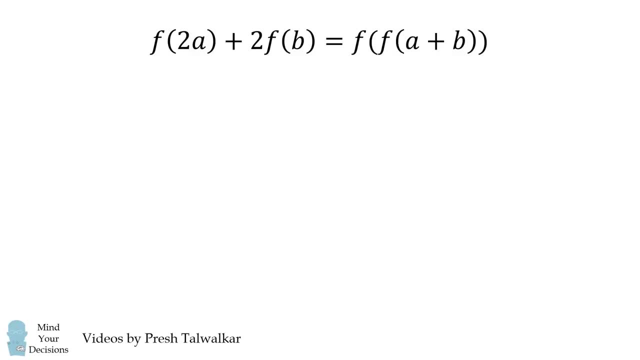 There may be other, easier ways, but this is just one way that I hope you'll understand. So we'll get started by trying some special values. Suppose A is equal to 0.. We'll take this equation and we'll substitute in: A is equal to 0.. 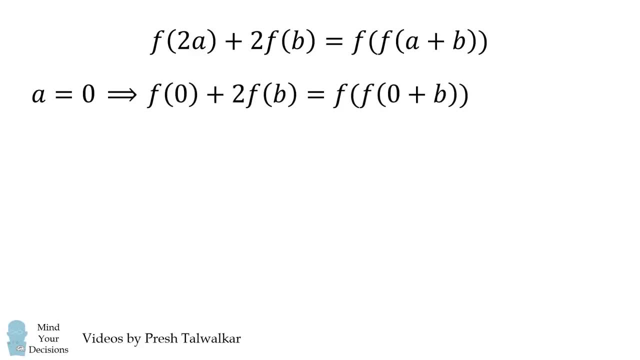 We get F of 0 plus 2 times F of B is equal to F of F of 0.. 0 plus B simplifies to be B. Next, we'll consider that this is true for all integers B. Therefore we can substitute the variable X here and say it's true for all integers X. 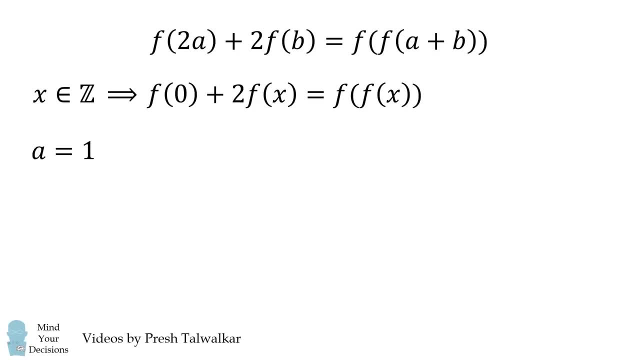 Now let's try. the special value A is equal to 1.. So we take our identity and then substitute: A is equal to 1.. 1 plus B will be B plus 1, because addition is commutative. We're now going to take this F of F of B plus 1 and simplify it. 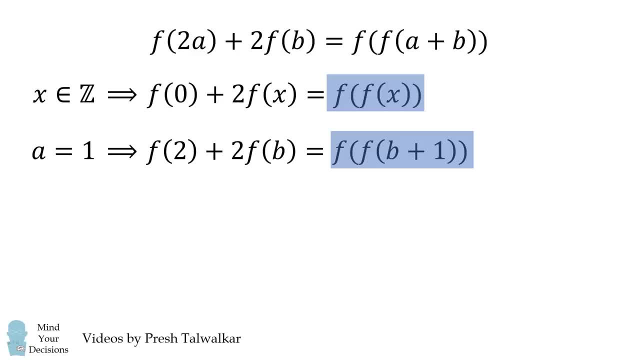 How can we do that? Well, look at our first identity. We have a composition of F of F of X, So we substitute in B plus 1 wherever we see X, and we end up with F of 0 plus 2 times F of B plus 1.. 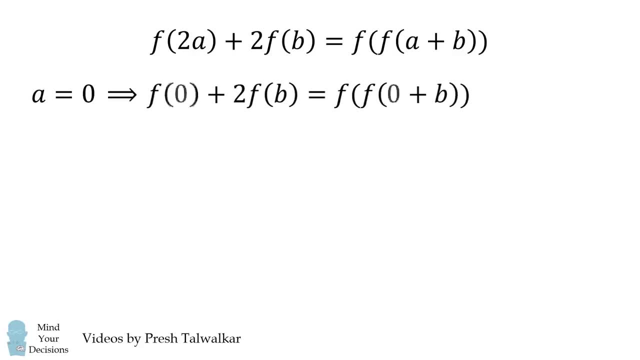 this equation and we'll substitute in: A is equal to 0.. We get f of 0 plus 2 times f of b is equal to f of f of 0.5.. We'll take this equation and we'll substitute in: a is equal to 0.. We get f of 0 plus 2 times f of b is equal to f of f of 0.5.. 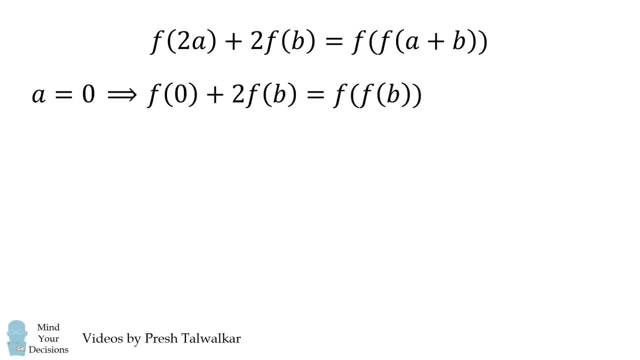 0 plus b simplifies to be b. Next, we'll consider that this is true for all integers b. Therefore we can substitute the variable x here and say it's true for all integers x. Now let's try the special value. a is equal to 1.. 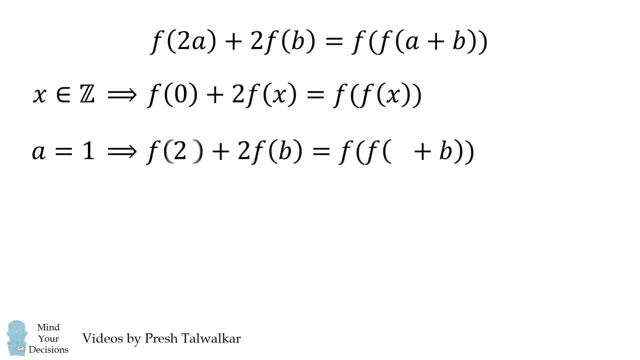 So we take our identity and then substitute: a is equal to 1.. 1 plus b will be b plus 1, because addition is commutative. We're now going to take this f of f of b plus 1 and simplify it. How can we do that? 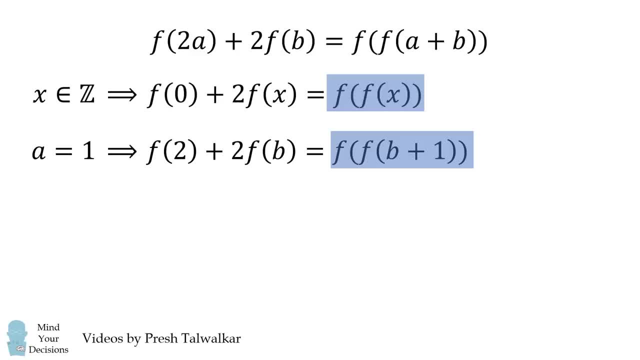 Well, look at our first identity. We have a composition of f of f, of x, So we substitute in b plus 1 wherever we see x, and we end up with f of 0 plus 2 times f of b plus 1.. So this will become another identity. Now recall that this is true for all integers b. So we'll substitute x here. 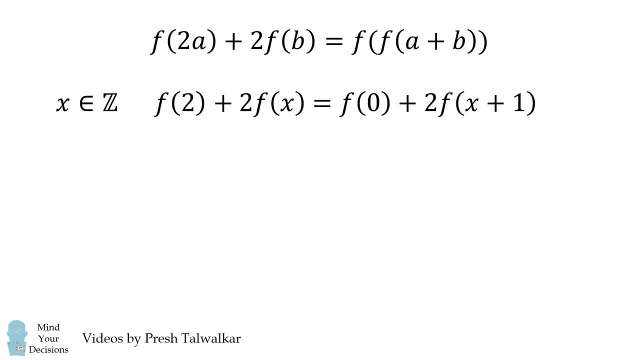 And we'll just write that it's true for all integers x. Now we're going to manipulate this equation. We have an x term on the left and a constant term on the right, So we'll switch them to the other side. We'll bring the constant term to the left side. 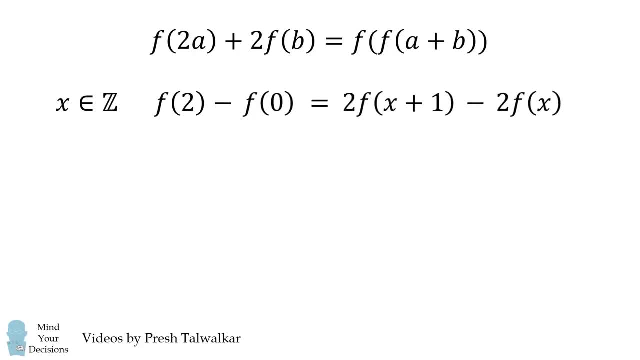 and the x term to the right side. Now we'll divide both sides of this equation by 2.. Notice: the right hand side of the equation will be the difference of consecutive terms. This is f of x plus 1 minus 1.. minus f of x. 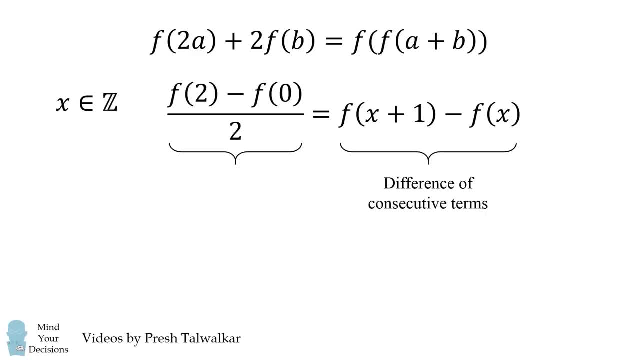 The left-hand side of the equation will be the value of the function at 2 minus the value of the function at 0, all divided by 2.. Therefore, this will be a constant value, and it's true for all integers x. 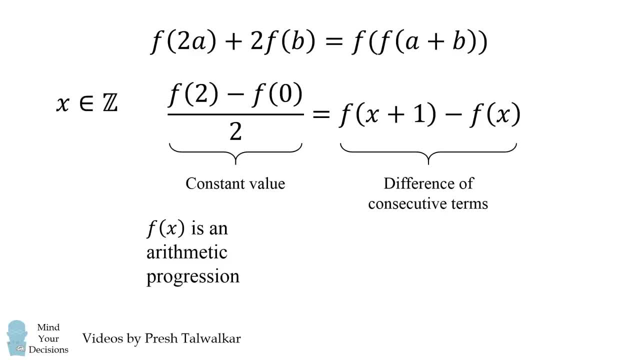 This means we have an arithmetic progression because the difference of consecutive terms will be some constant value. This means f of x can be written as the linear equation m times x plus n. We now take this form and substitute it back into the original equation. 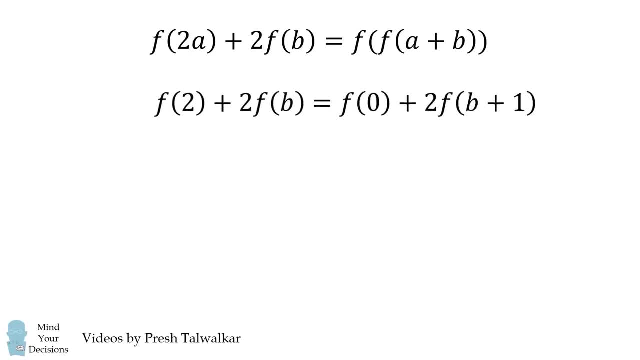 So this will become another identity. Now recall that this is true for all integers B. So we'll substitute X here And we'll just write that it's true for all integers X. Now we're going to manipulate this equation. We have an X term on the left and a constant term on the right. 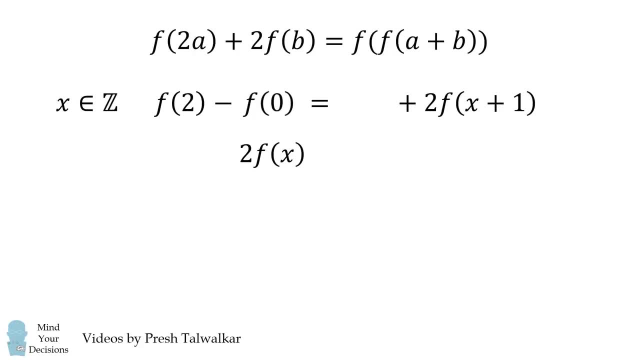 So we'll switch them to the other side. We'll bring the constant term to the left side and the X term to the right side. Now we'll divide both sides of this equation by 2.. Notice, the right-hand side of the equation will be the difference of consecutive terms. 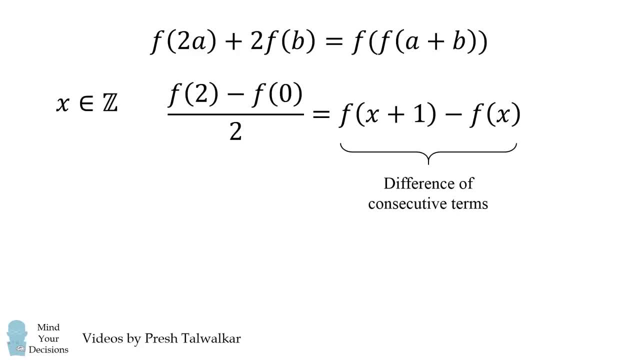 This is F of X plus 1 minus F of X. The left-hand side of the equation will be the value of the function at 2 minus the value of the function at 0, all divided by 2.. Therefore, this will be a constant value, and it's true for all integers X. 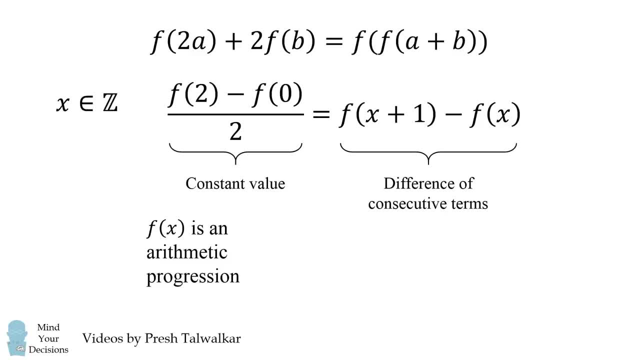 This means we have an arithmetic progression because the difference of consecutive terms will be some constant value. This means F of X can be written as the linear equation M times X plus N. We now take this form and substitute it back into the original equation. 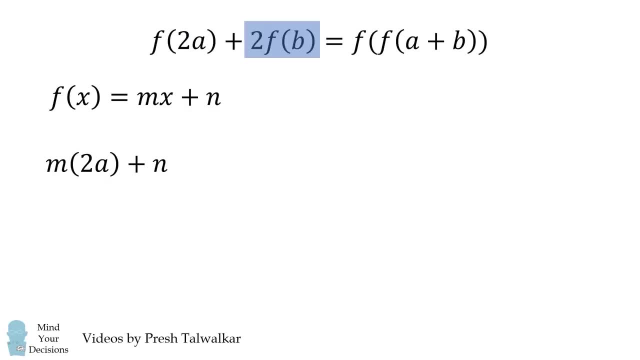 We start with F of 2A, Then we go to 2 times F of B And finally we have a composition. So first let's do F of A plus B, Then let's do another evaluation of the function. When we do that, we end up with the following equation: 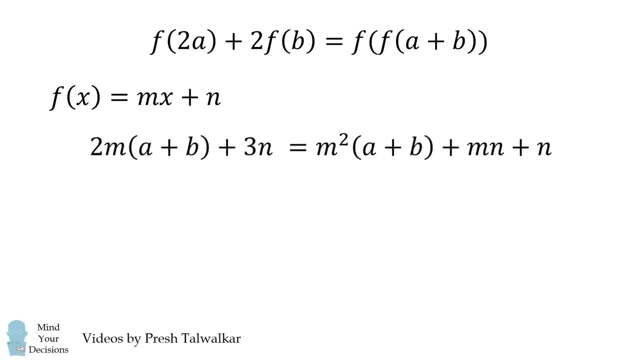 We simplify both sides. and now how are we going to figure out M and N? We're going to match coefficients of like terms. So here we have the term A plus B on the left and A plus B on the right, And this has to be true for all integers, A and B. 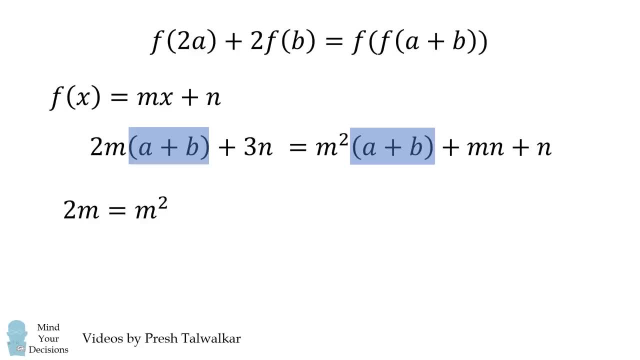 The only way this is true is if we match the coefficients 2M and M squared. Now we also match the constant terms. So we have: 3N is equal to M times N plus N. We have a system of equations. We're going to solve this by considering each case. 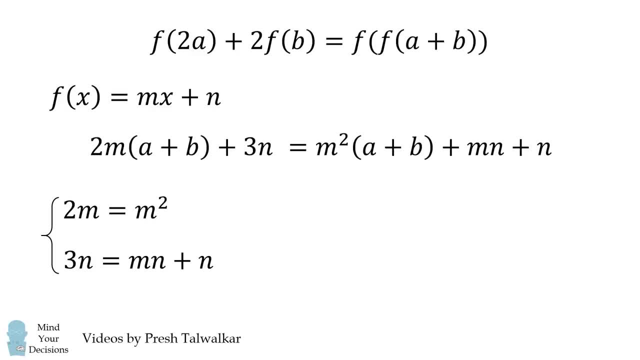 So how do we solve? 2M is equal to M squared. Well, one solution is: M is equal to 0.. We're going to substitute that into our second equation. We have: 3N is equal to N, and that's only true if N is equal to 0.. 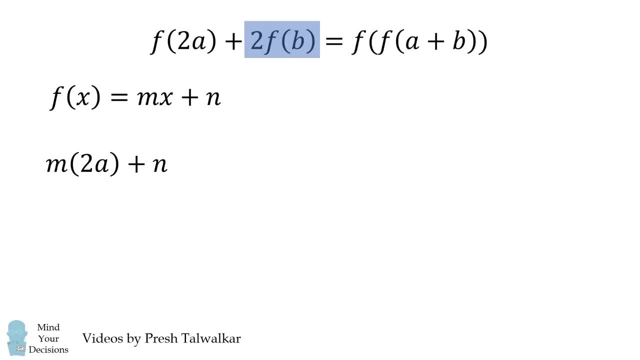 We start with f of 2a, then we go to 2 times f of b and finally we have a composition. So first let's do f of a plus b, then let's do another evaluation of the function. When we do that, we end up with the following equation: 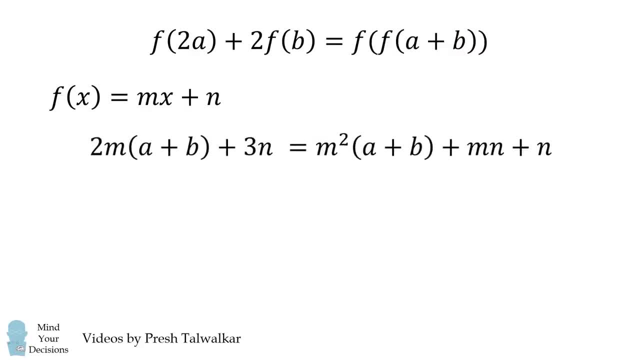 We simplify both sides. and now how are we going to figure out m and n? We're going to match coefficients of like terms. So here we have the term a plus b on the left and a plus b on the right, and this has to be true for all. 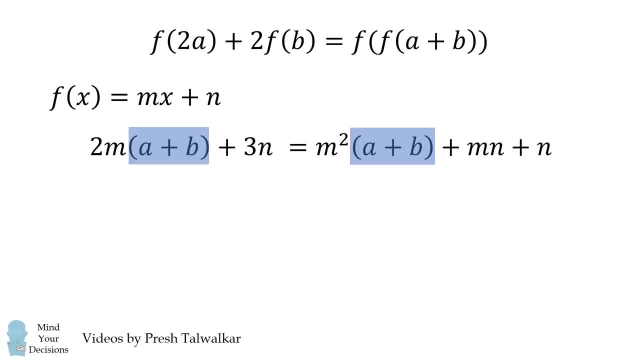 integers a and b. The only way this is true is if we match the coefficients 2m and m squared. Now we also match the constant terms, so we have: 3n is equal to m times n plus n. We have a system of equations. 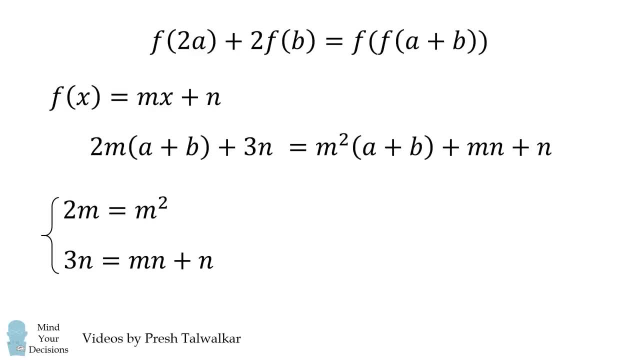 We're going to solve this by considering each case. So how do we solve? 2m is equal to m squared. Well, one solution is: m is equal to 0.. We're going to substitute that into our second equation We have: 3n is equal to n, and that's only true if n is equal to 0.. 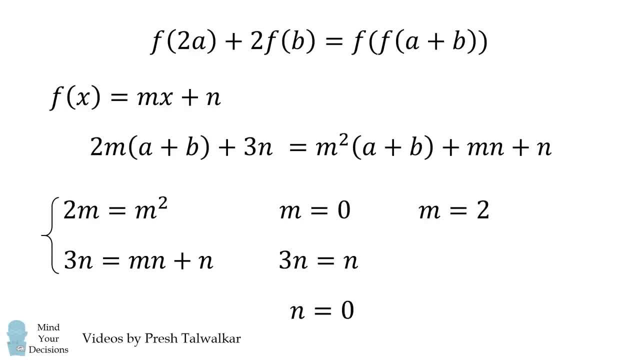 The other possibility is that m is equal to 2. In this case we substitute in and get: 3n is equal to n, so n can be any integer, And we now have two possibilities for our solution. One will be: f of x is equal to 0, and the other is that f of x is equal to 2 times x plus n. 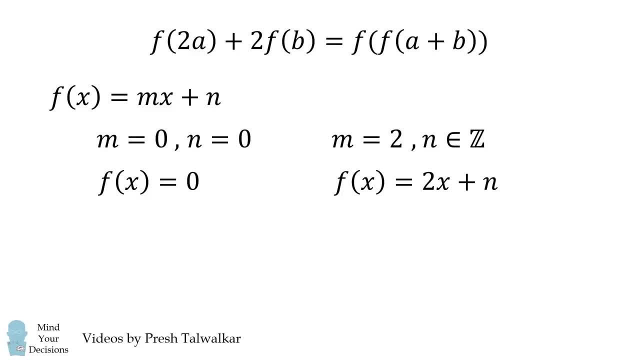 for some integer n in z. We want to verify that these actually are true and substitute them back into our original equation. We can do that and we'll see that we'll get equality for both cases. Therefore, these are the only solutions. 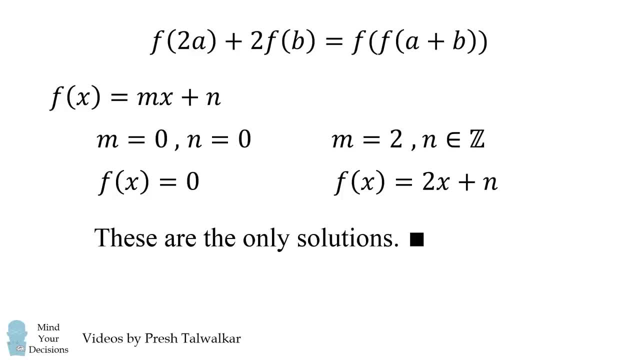 Either f of x is identically 0, or f of x is equal to 2 times x plus n for some constant n. I hope this video gave you some sense of how to solve an Olympiad problem and I hope it gave you some idea of how challenging these problems are.